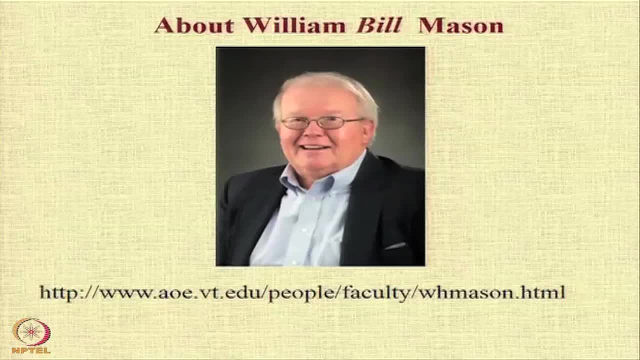 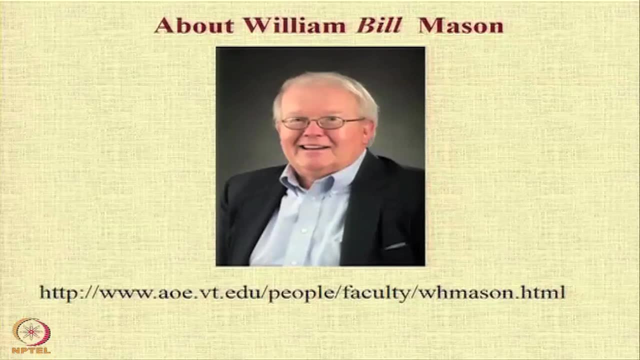 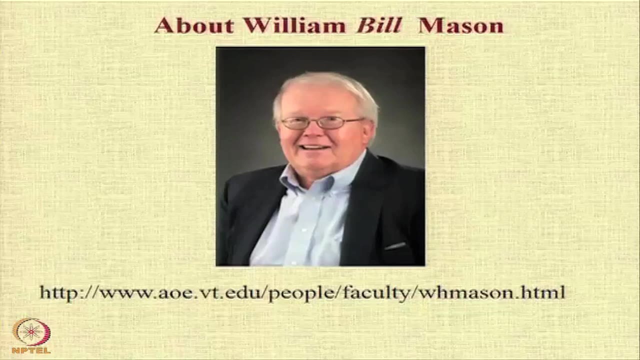 design at Virginia Tech and also is a very established aerodynamicist. Those who want to know about Bill Mason should go to this website. Bill Mason is associated with collecting and keeping a large amount of data related to aircraft design: Several codes. several interesting reports are available on his site And he was among 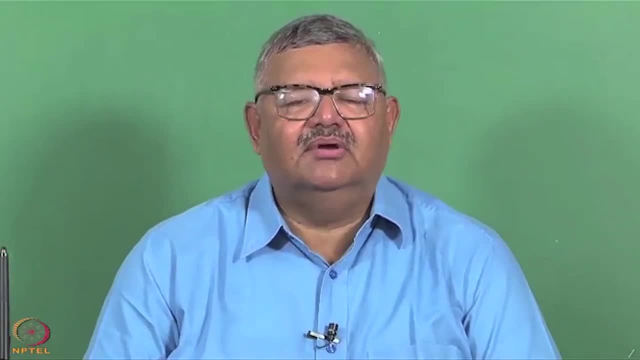 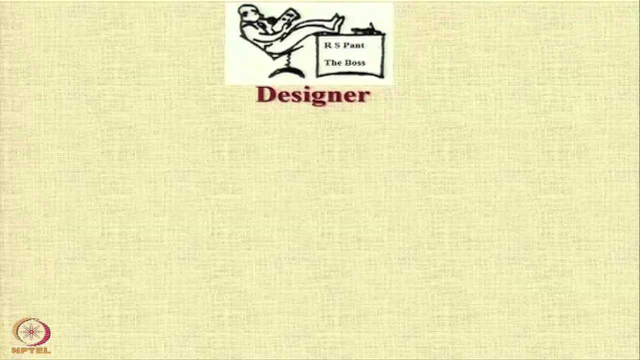 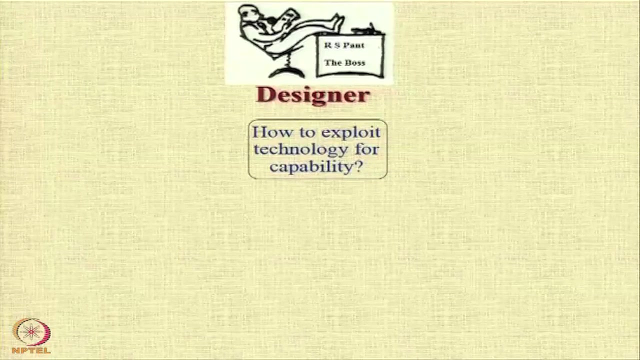 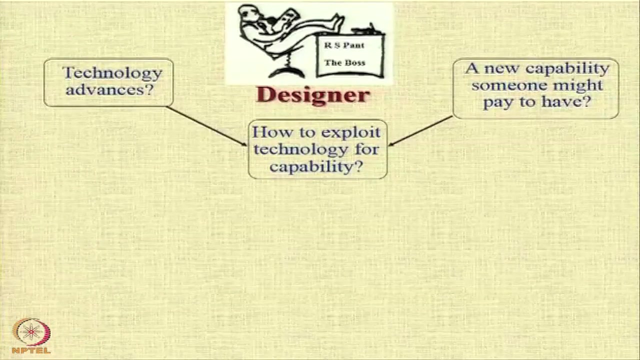 the first people to make information publicly available on his website. So you have a person who is a designer, who is the chief, he is the boss, And his main area of interest or concern is: how do we exploit the technology for generating new capability? 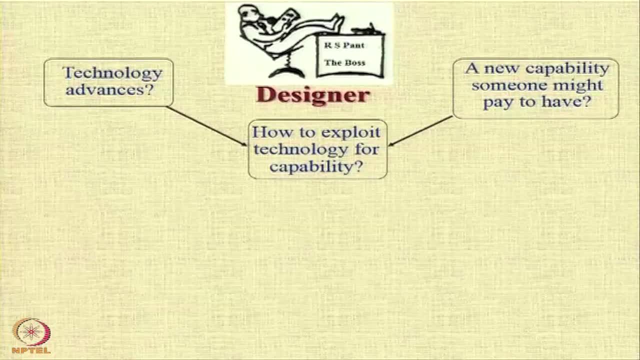 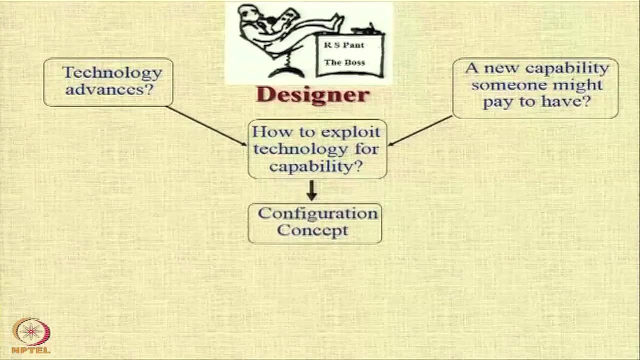 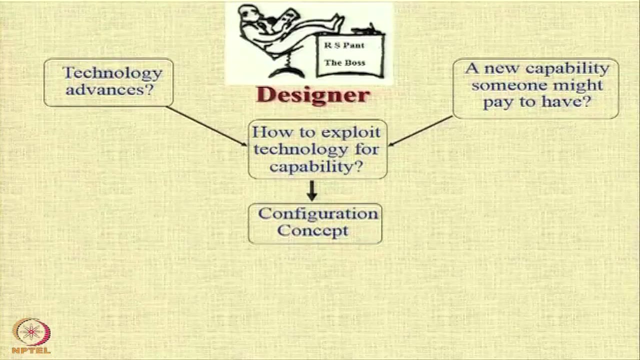 Shall we use a new capability that someone might pay to have, or shall we have a look at the advances in technology and see if we can apply them to meet the customer requirement? So, keeping these two in mind, the design team I have shown here as an individual, but 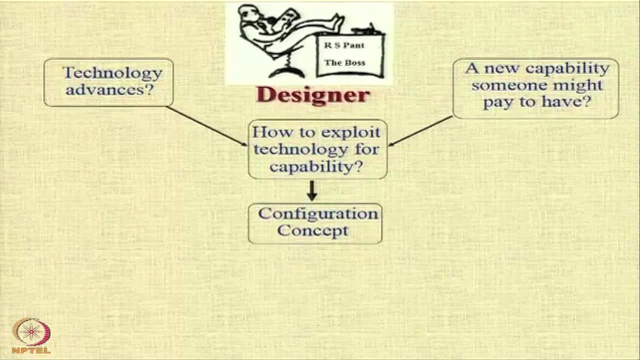 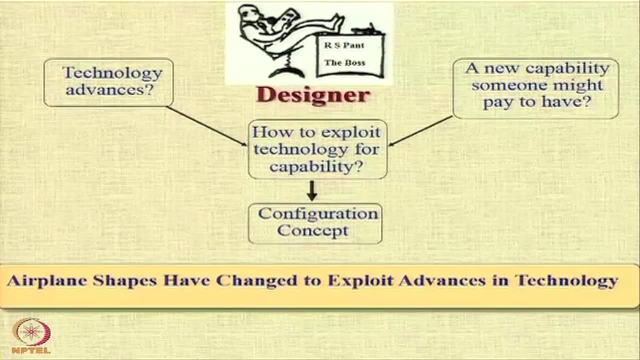 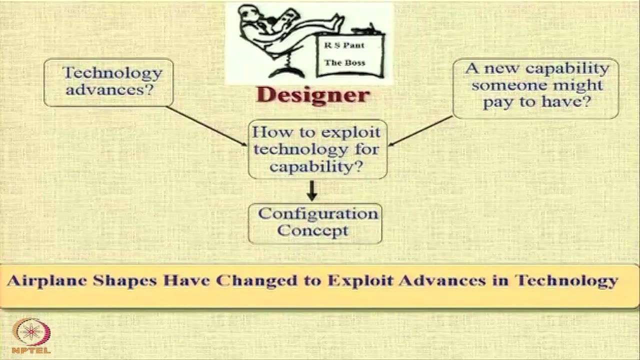 in real life it is not an individual. In real life it is not an individual, It is actually a team. They come up together with a configuration concept- And there is an interesting note that shapes of the aircraft have changed over the years- to exploit the advances in 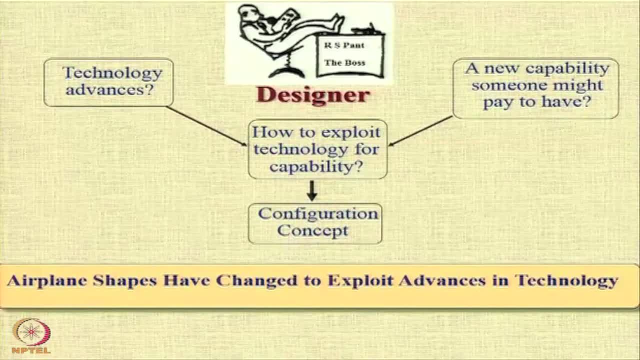 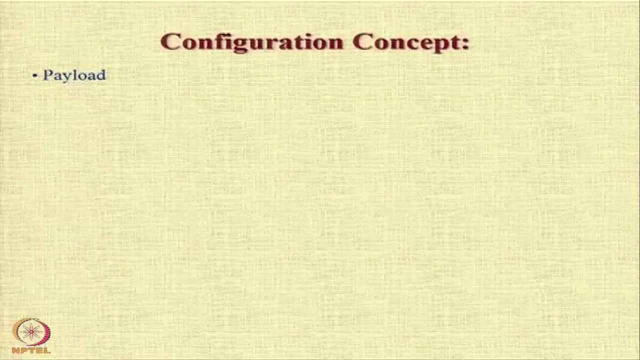 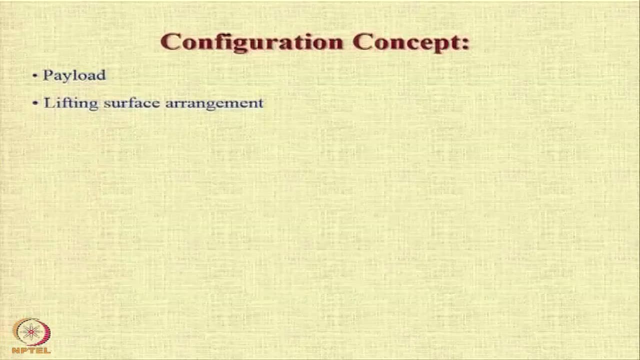 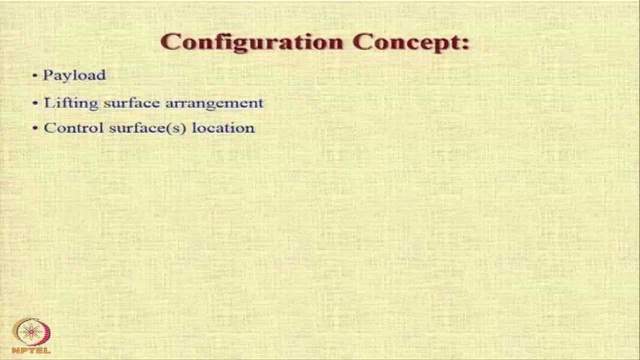 technology, And this statement will be elaborated in detail in the next few slides. When we talk about the configuration concept, we have to understand that we are looking at how to locate items like the payload. What kind of lifting surface arrangement we need to use? Do we have a control surface or many control surfaces, and what is their? 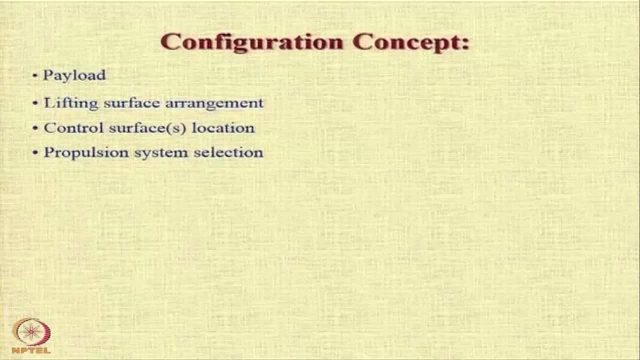 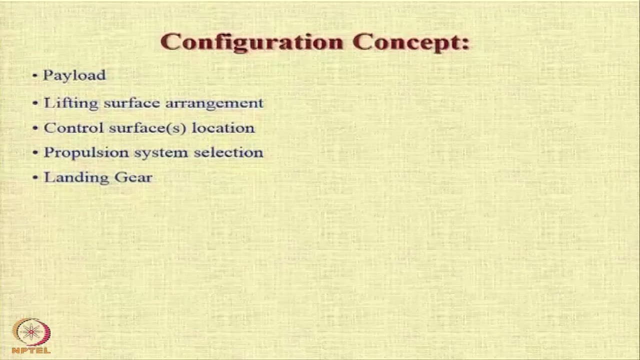 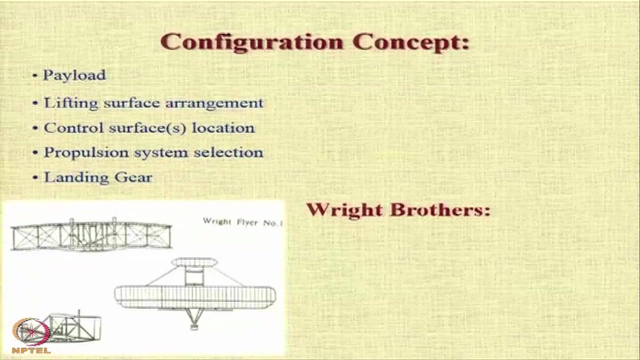 location. We have to decide what kind of propulsion system we will use And we have to also decide if we have a landing gear and what type and roughly what kind of a landing gear layout. Let us see. Let us start by looking at the first successful aircraft which the Wright brothers had developed. 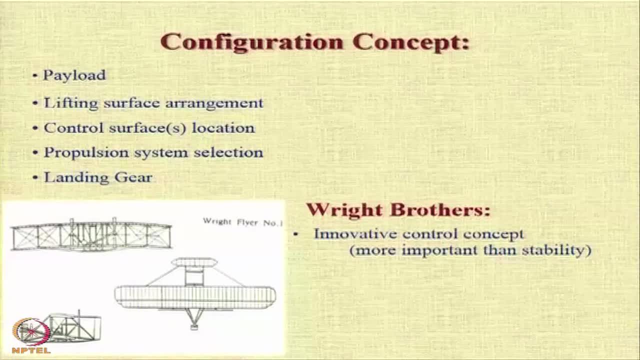 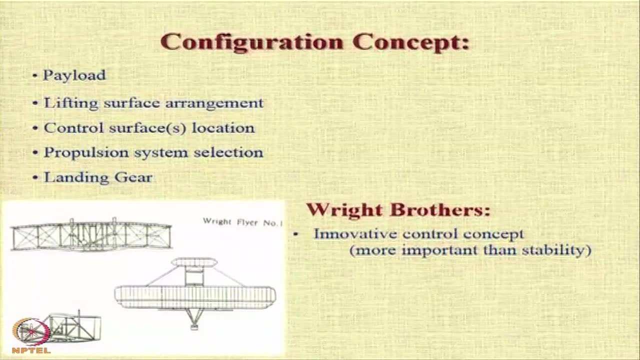 What were the key configurational aspects of this particular aircraft? First, they went for a very innovative control concept. They were more concerned about control than about stability, So that is why they have used canards. They were very accomplished flyers and they were trying to achieve a milestone And using the canards, they were using the 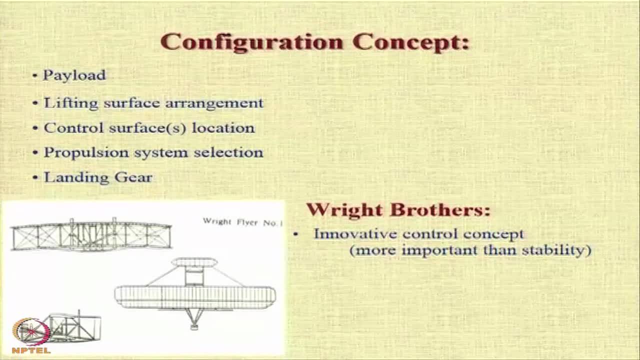 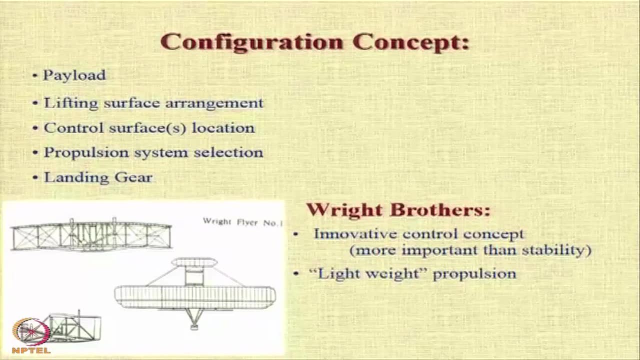 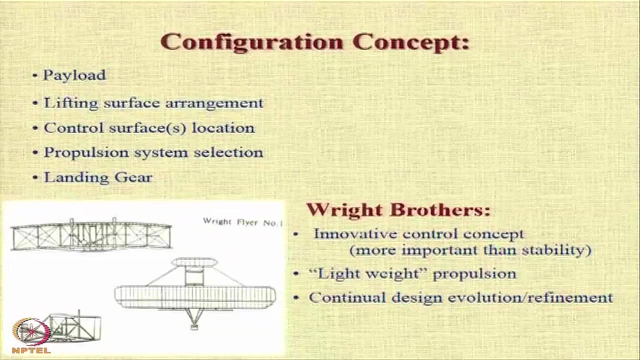 canards that were in the air and the canards that were in the air And they were trying using their piloting skills. they were able to successfully achieve flight. They were also successful partly because they were able to integrate a very lightweight propulsion system onto their aircraft and their design was a continual improvement and evolution. it was 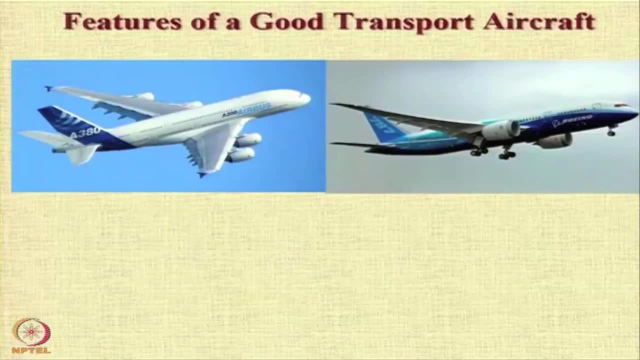 not overnight. Let us look at what are the features of a good transport aircraft, and this. this slide shows one aircraft from the Airbus stable and one from the Boeing stable. They all, they both look quite similar, except one of them is twin engine, the other is with. 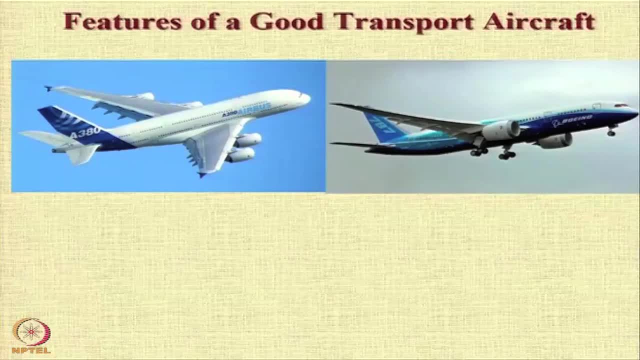 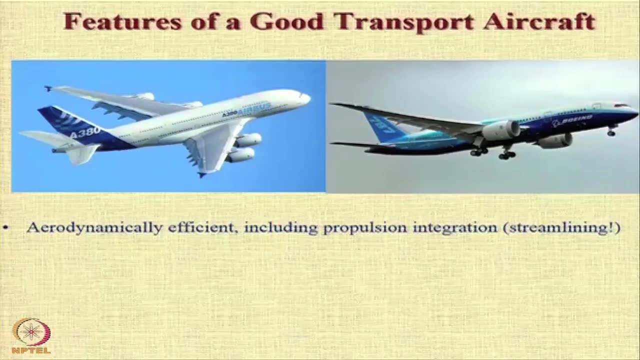 four engines, but both of them share some standard good features. First of all, a good transport aircraft has to be aerodynamically efficient, and when I say this, I always also mean integrating the propulsion system in such a manner that the aerodynamic efficiency is not compromised, and this is achieved by what is called as streamlining. 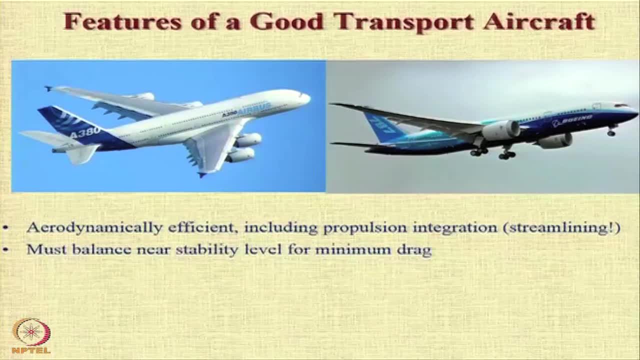 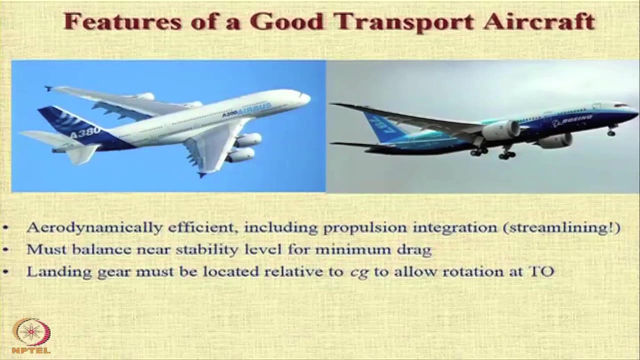 So a good transport aircraft should be properly streamlined. It must balance near the stability level for minimum drag. If it balances at some other location then the drag is going to be higher because the trim drag, which is one component of the drag, We will have a 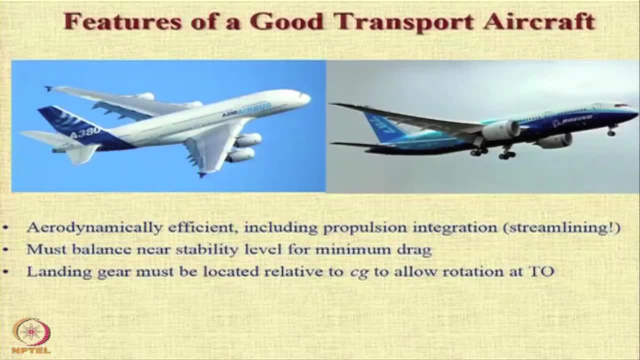 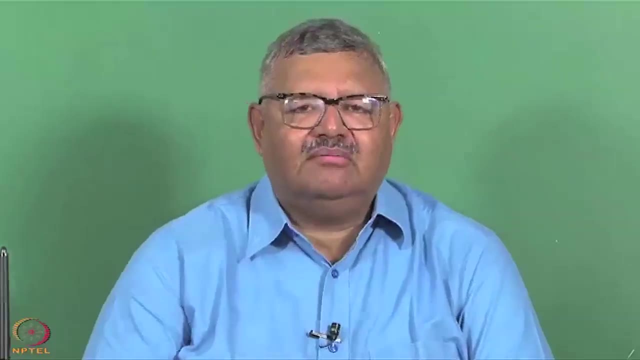 look at drag estimation and drag components little bit later There. I will elaborate this point little bit further. In a good transport aircraft the landing gear must be located relative to the center of gravity. This should be done in such a manner that the aircraft can easily rotate. 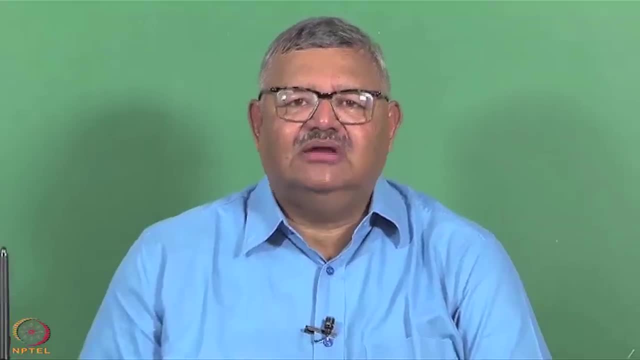 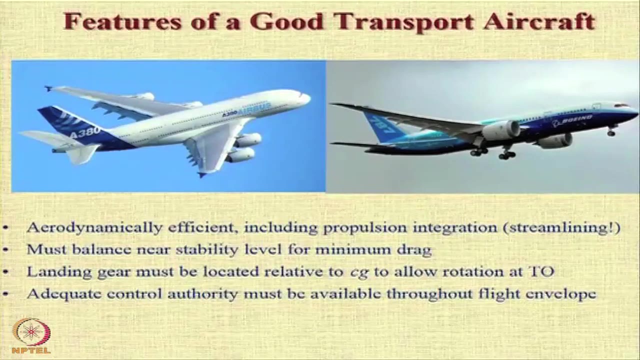 during the takeoff, Otherwise the takeoff distance is going to be reduced, It is going to be large or you will need a very large size control surface Throughout the flight envelope or throughout the height and velocity envelope in which the aircraft has been cleared to operate. we must have adequate control authority so that there is 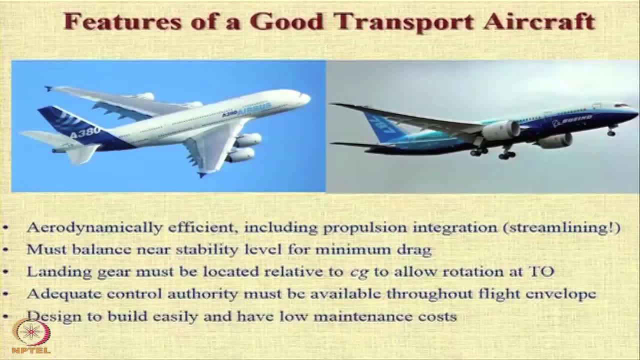 no chance of the aircraft entering into any area of instability. Also, as we mentioned right in the beginning, Design is good if it can be built easily and in large numbers so that it becomes affordable, and also it should have low maintenance costs so that the operating costs are minimized. 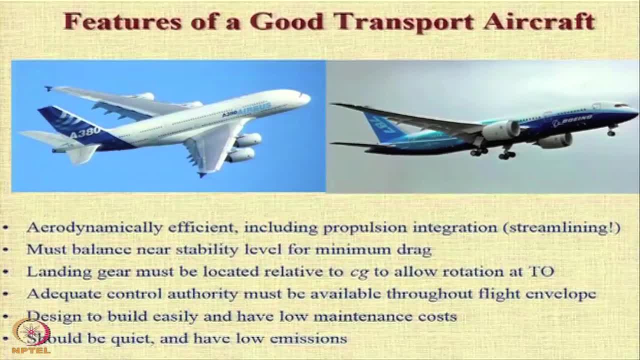 And in modern days an aircraft has to be a good neighbor. It has to be able to operate in the our environment without much disturbance, So it should be quiet and it should have low emissions. So these six points are the hallmark of a good transport aircraft. and the configuration. 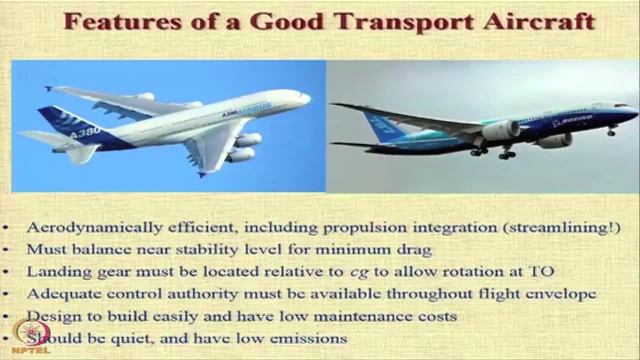 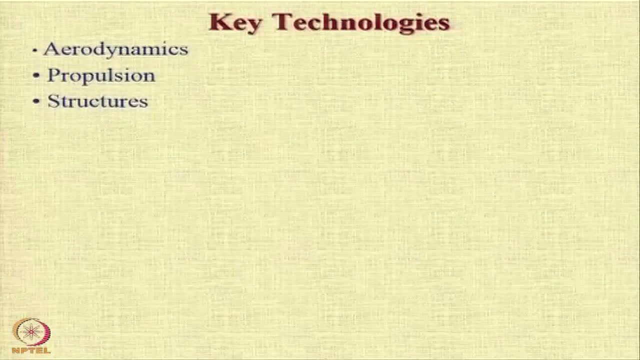 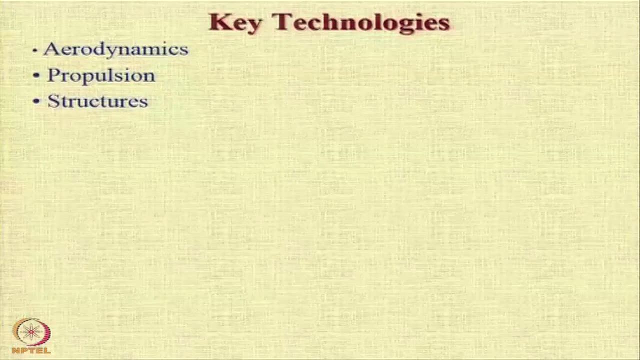 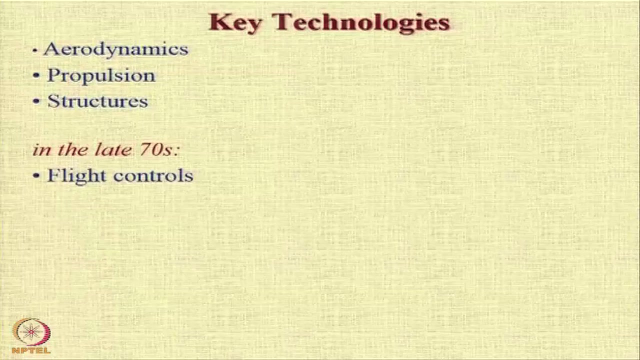 of the aircraft should be chosen. to try and achieve a balance in these six points, Let us look at the key technologies that are used in designing an aircraft: Aerodynamics, propulsion and structures. These are very well known technologies. about these we study. In the late 70s, flight controls as a technology began emerging as a huge role player In the 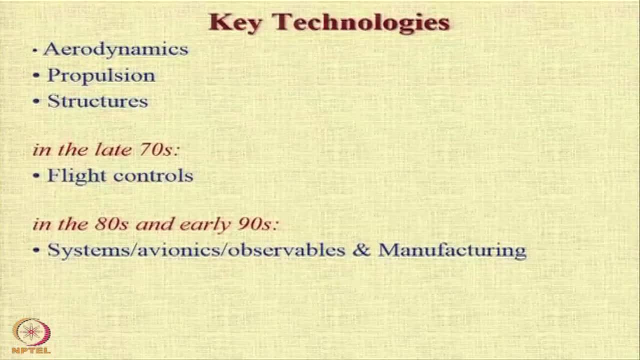 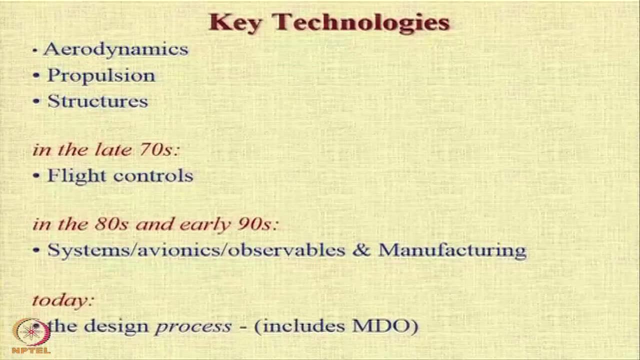 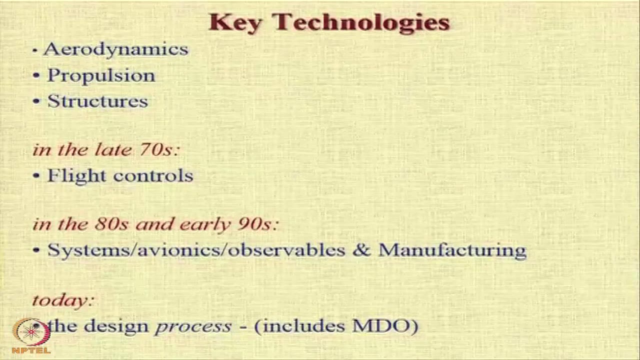 80s and early 90s we started looking at systems, avionics and observables and manufacturing technology. manufacturing techniques became very important And today the design process itself is the key technology. We have today, a technology called as multidisciplinary. 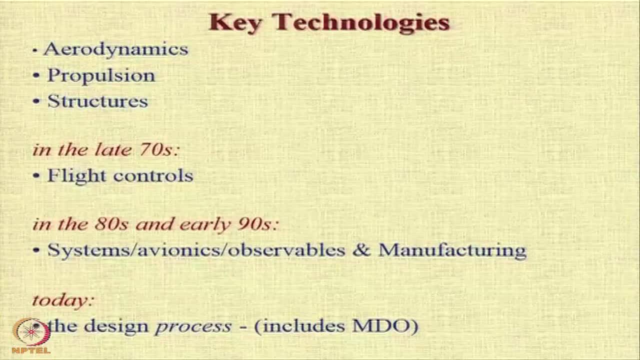 design optimization, which is used in a laboratory design approach. So we have a range of technologies. So we have a wide variety of technologies like Porche, Scentron, Aero-Aesthetic and all the to conceive and design the aircraft, keeping in mind the interaction between various disciplines. 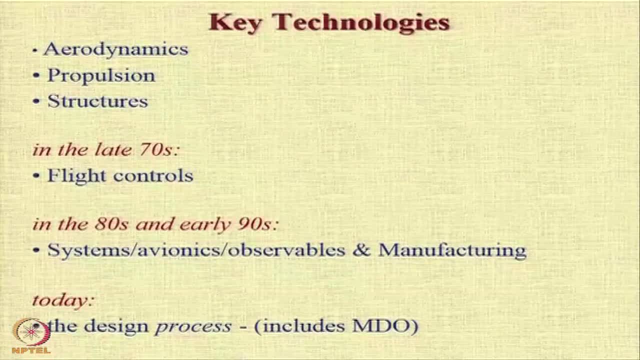 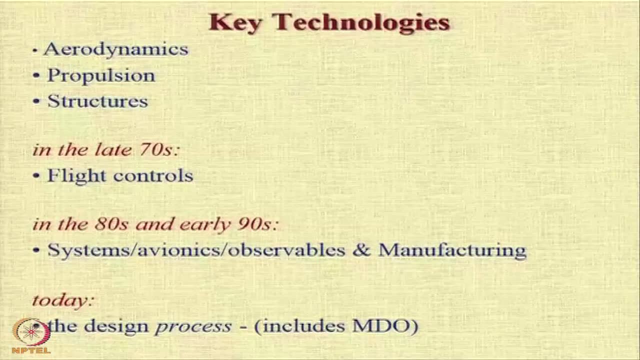 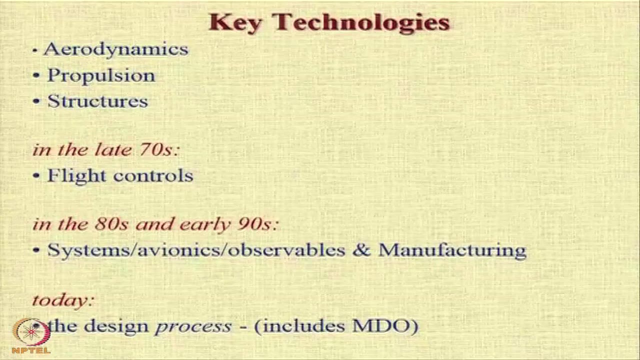 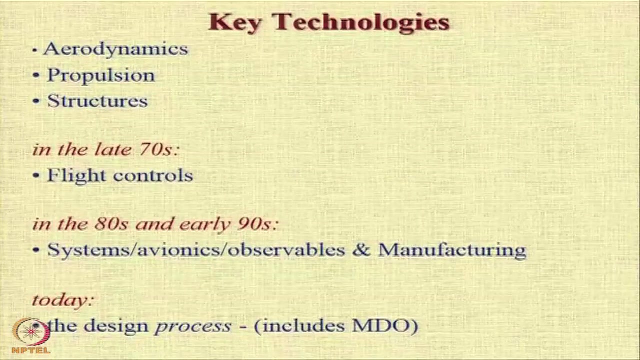 and trying to achieve excellence and efficiency right from the beginning, And to do this, the various interactions between disciplines have to be captured, and hence we have to look at a concurrent approach and that is very well amenable to analysis using the MDO techniques. So today, aircraft design is mostly driven by the MDO technology available. 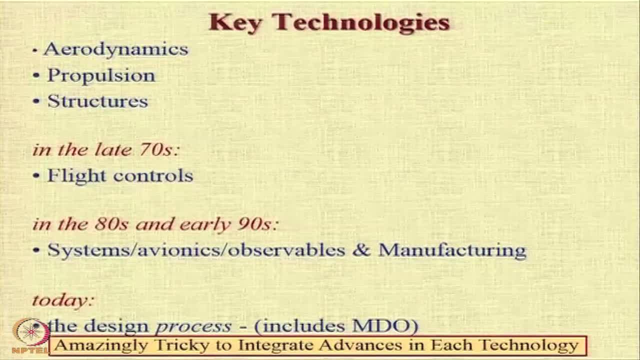 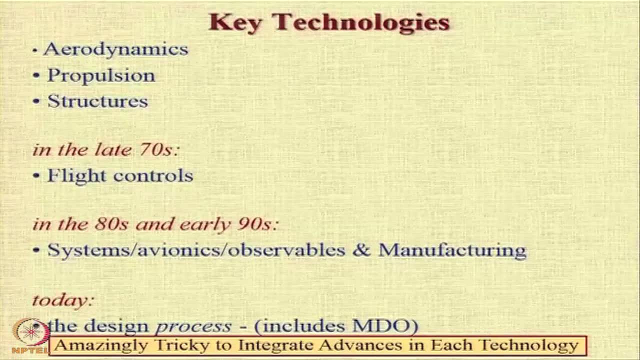 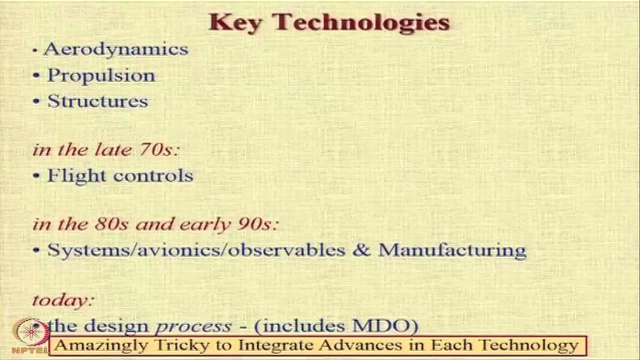 Now, it is not very easy to integrate advances in each technology into this multidisciplinary environment, and sometimes individual technological developments can cause a lot of problem or issues when they have to be integrated. Let us look at what is meant by a B-project selected as B-project or a pre-project, and what are those are the factors associated with that best execution. 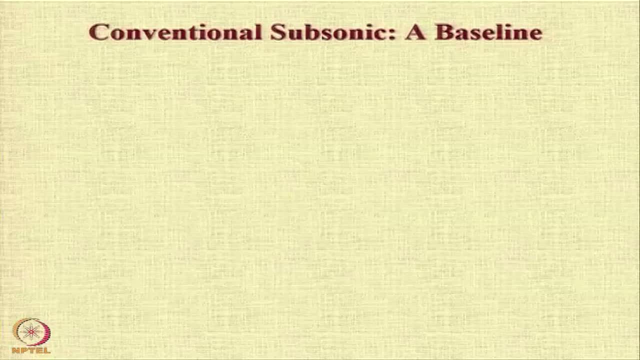 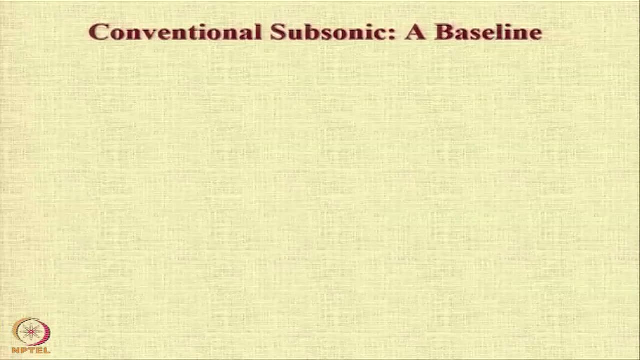 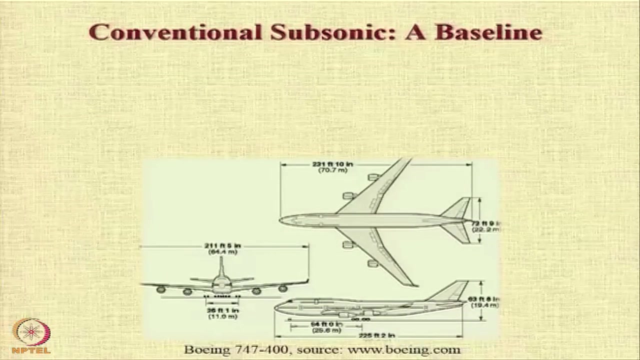 baseline aircraft, because any innovation or any new configuration will be considered with respect to this particular baseline. So for a subsonic transport aircraft, you have a baseline which was first suggested by the Boeing company in the form of Boeing 747.. So what are the features? We distribute the payload around the center of gravity. So 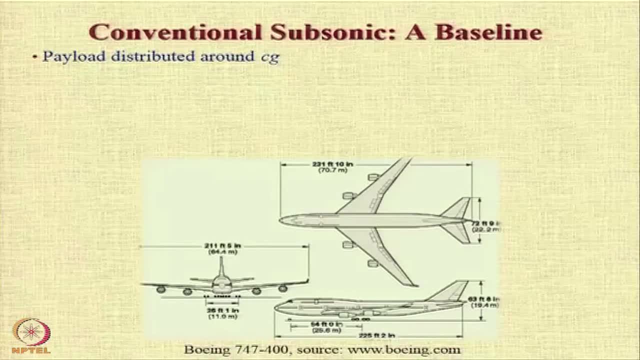 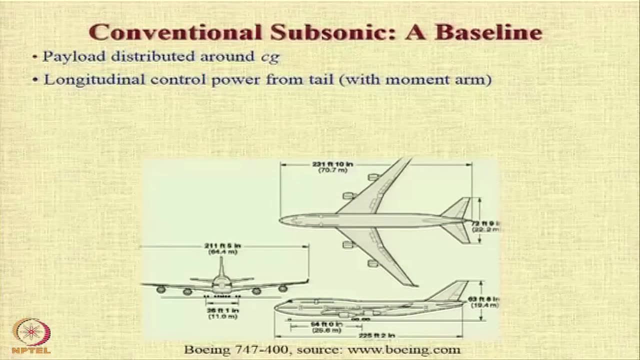 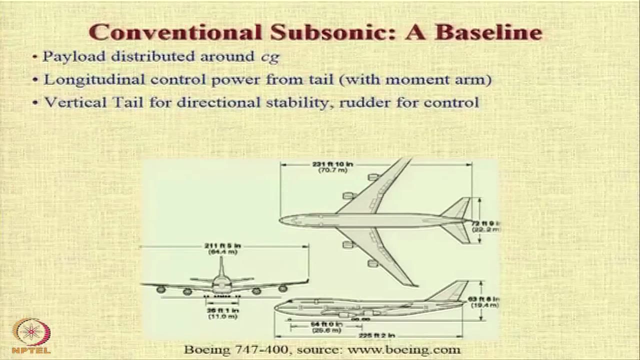 some part of the payload is ahead of the center of gravity, some part is behind and we try to maintain the CG. We provide longitudinal control using a conventional tail mounted behind and using a moment arm we provide the required control power. We provide a vertical tail for giving a directional stability and rudder for control And 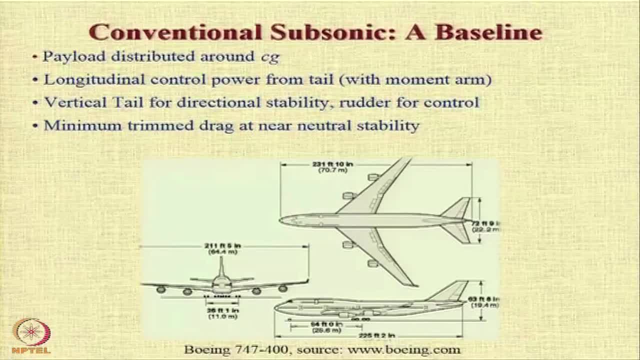 we try to fly the aircraft such that the trimdraft drag is minimum near the location or near the stability level at which we want it to fly. Trimdrag is caused because of the drag due to the control surfaces, which are deflected in order to trim the aircraft or in order to create a situation where the net moment acting on the 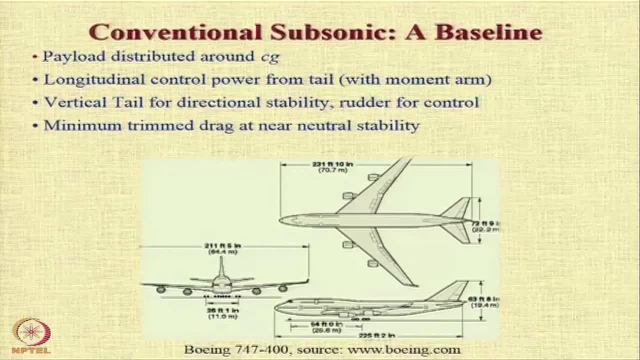 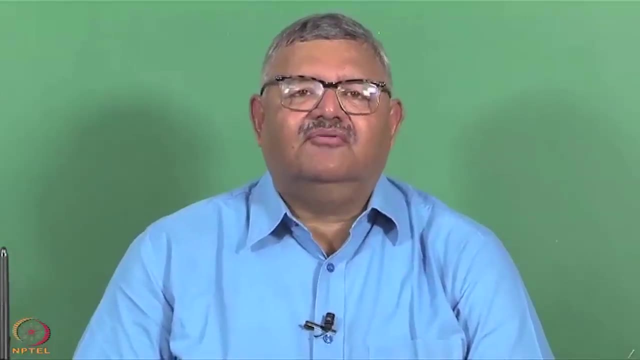 aircraft is 0 about the center of gravity And larger the deflection of control surfaces needed, larger will be the drag because of them and that will continue throughout the flight and hence it is going to contribute a large amount to the drag And hence it is important that the aircraft 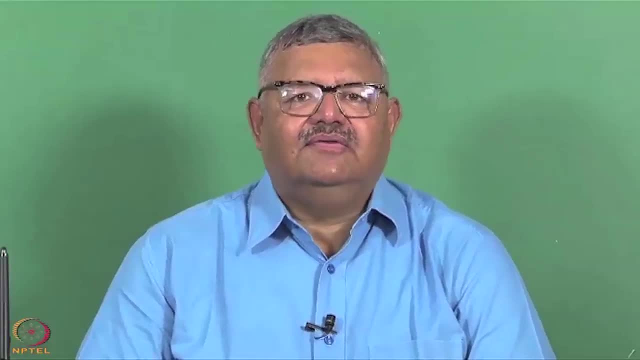 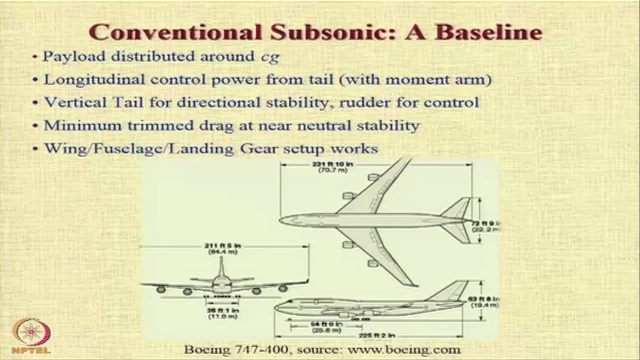 should be able to trim at little or no deflection of the control surfaces, And the standard setup that works for a conventional subsonic aircraft is the wing fuselage landing gear combination as shown in this figure. So any departure from this configuration for a subsonic transport aircraft. 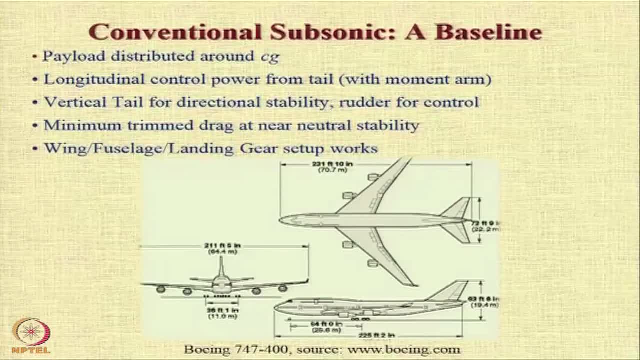 can be considered as a deviation or a variation configuration And there should be a pretty solid reason to do that. We are not saying that all transport aircraft look like this and should look like this. We are just saying that there has to be a solid reason to depart from this particular look. 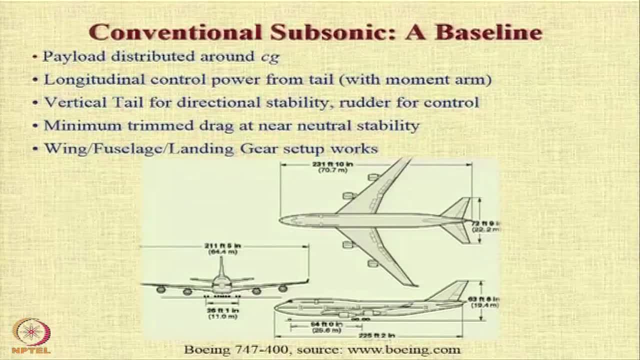 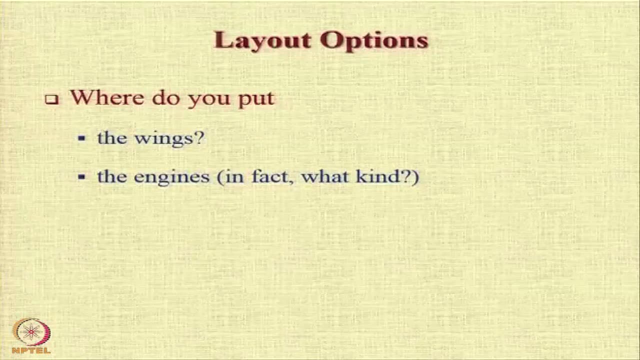 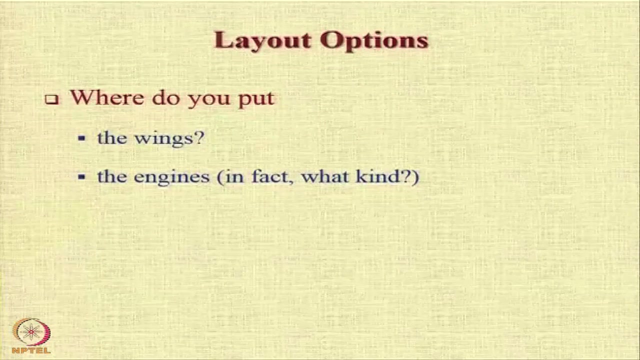 Because, over the years, the experience of designers have resulted in this kind of a configuration as the base. But, having said that, there are several options available to the designer for the layout. Layout stands for the relative location of the various major assemblies, like the wing, fuselage, tail, etc. So where do you put the wings? Do you put the wings ahead? 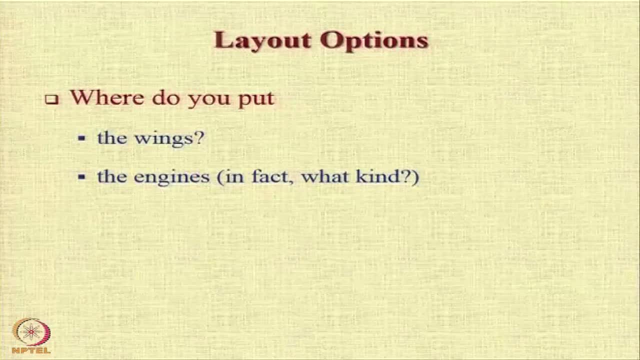 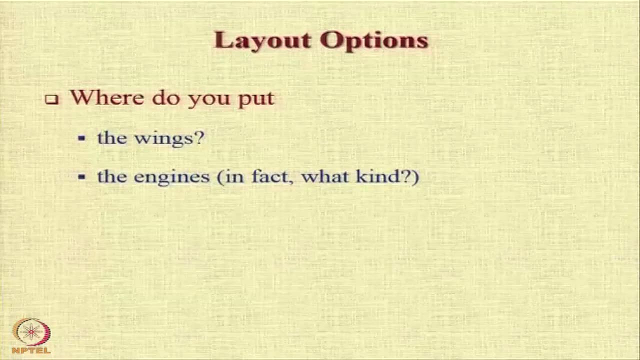 in the fuselage or behind? Do you put them above the fuselage or below, Or do you put it through the fuselage? Where do you put the engines? In fact, what kind of engines do you use And where do you put them? Do you put them below the wing, above the fuselage? 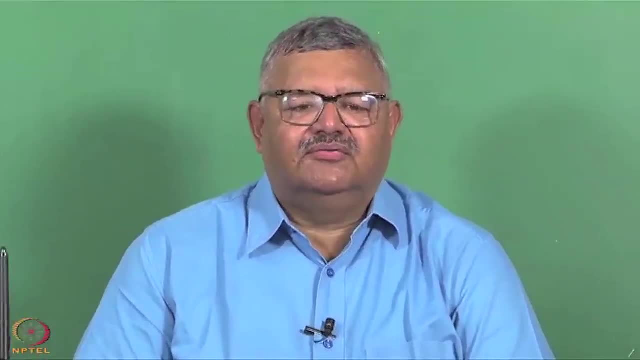 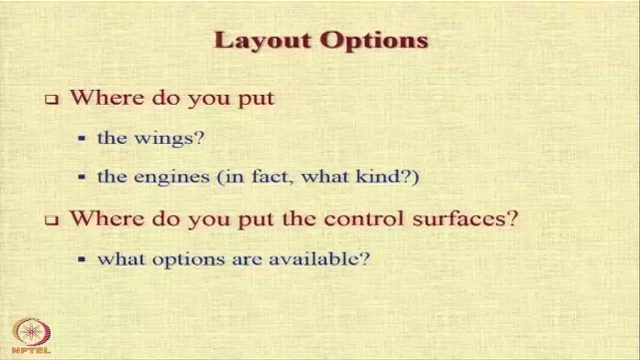 above the wing, on the front of the fuselage, on the rear of the fuselage, On the vertical tail- all these choices are available. Where do you put the control surfaces and what options are available for the control surfaces? And we have to be very careful that we should. 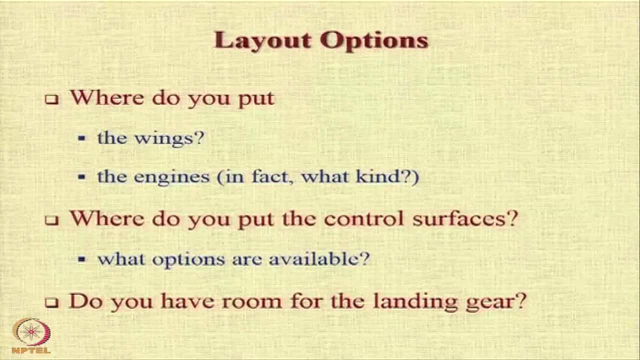 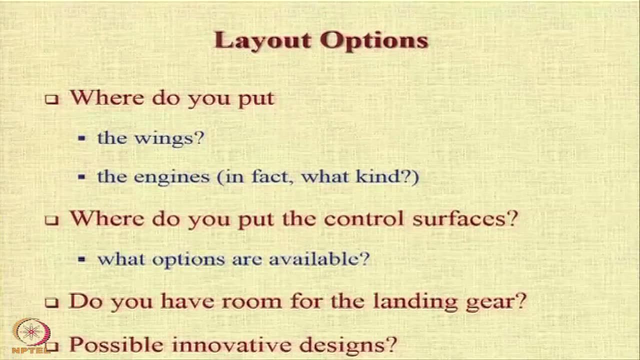 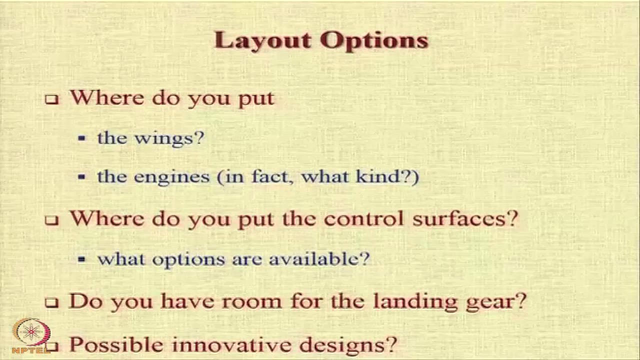 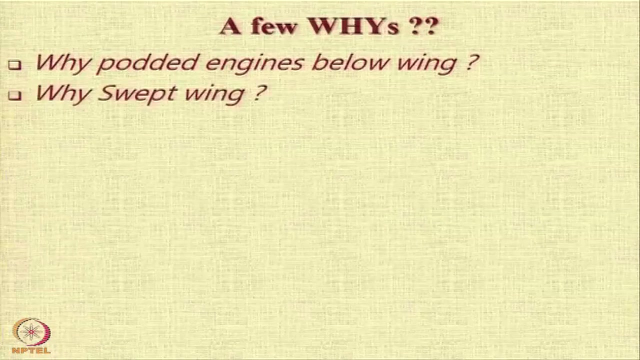 have sufficient room for landing gear, because landing gear is a necessary requirement for any large transport aircraft, And can we look at possible innovative designs to get improved manoeuvre or to meet some of the requirements which may not be possible to be addressed using the conventional baseline? At this point we start looking at questions that arise in the 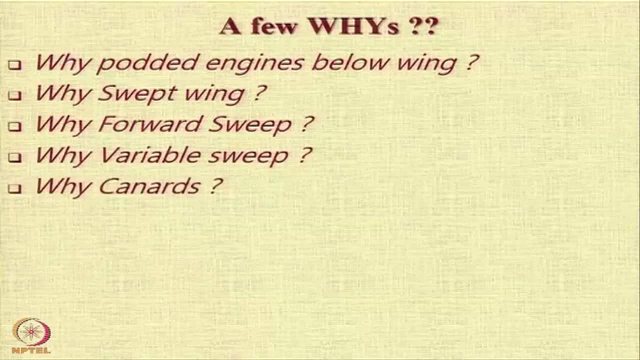 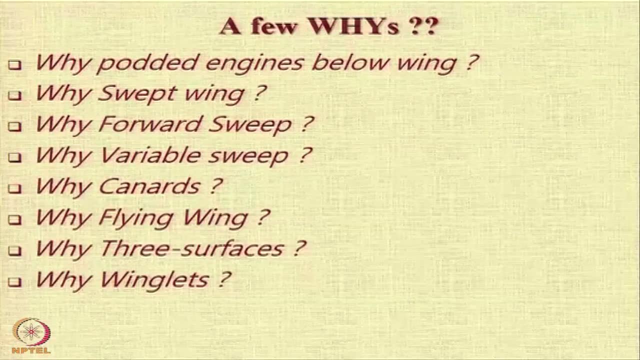 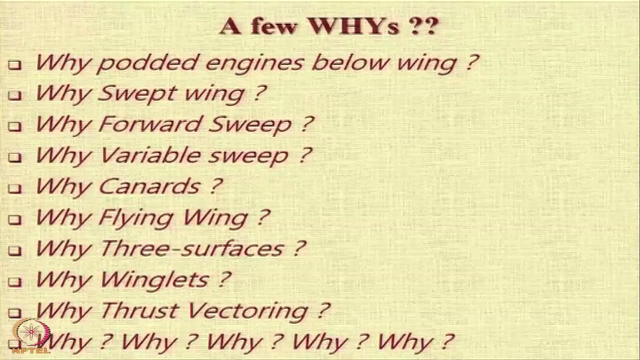 minds of a student about why we have a particular kind of a feature. Why do we have podded engines below the wings? Why do we have a swept wing? Why forward sweep? Why variable sweep? Why canards? Why flying wing? Why winglets? Why three surfaces? There are so many questions and there is a reason. 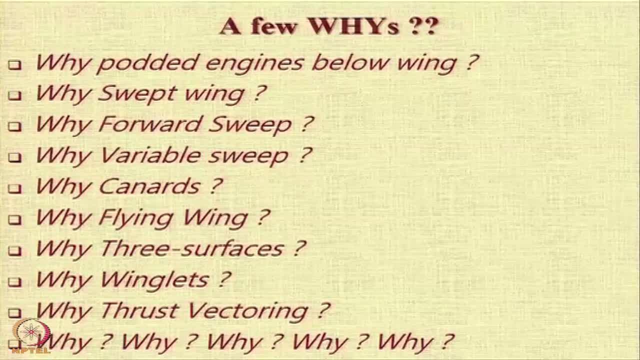 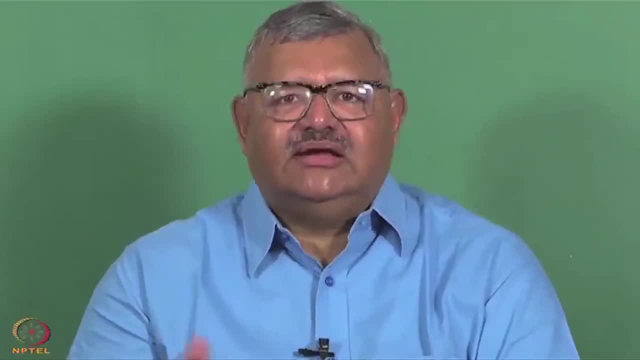 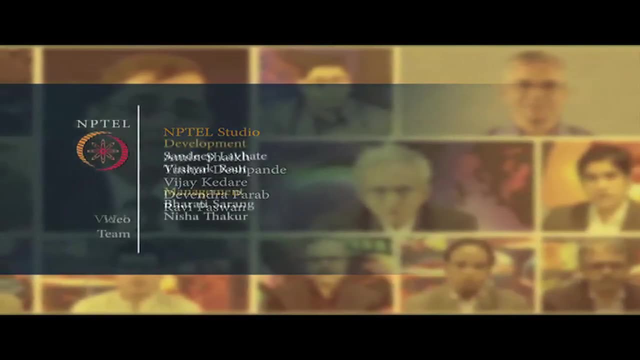 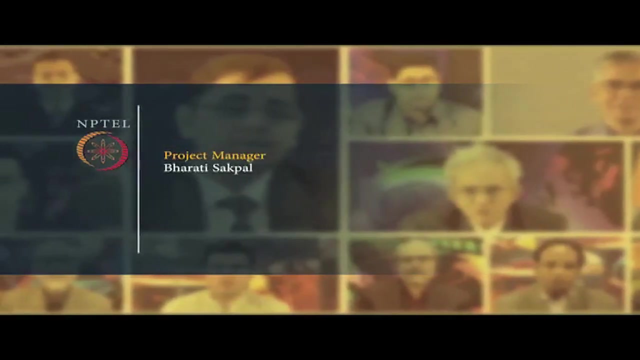 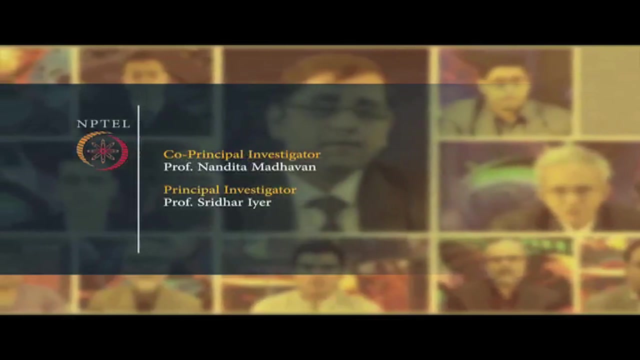 and a logic for each of these choices that the designer or a design team makes in the layout. Thanks for your attention. We will now move to the next section. Thank you.